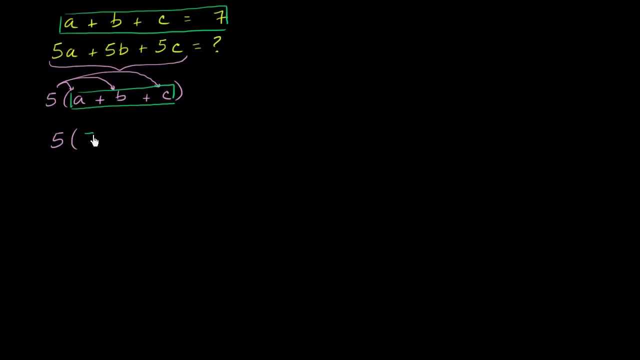 I think you see where this is going. now is 5 times 7. And now this becomes pretty straightforward: That's going to be equal to 35. Let's do one more of these and this is going to be a little bit more involved, but hopefully you see the same idea. 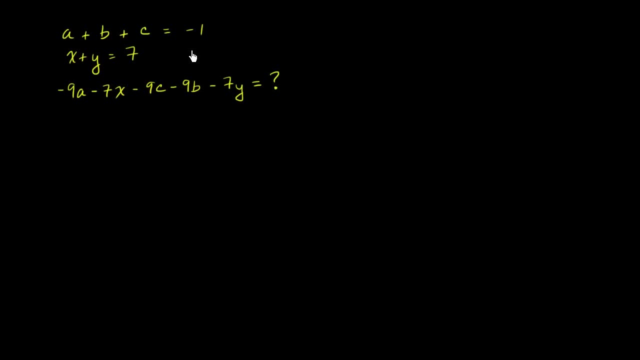 So we're told that a plus b plus c is equal to 7.. So 5 times a plus b plus c is equal to 35.. a plus b plus c is equal to negative 1.. And we have two more variables here, We're told. 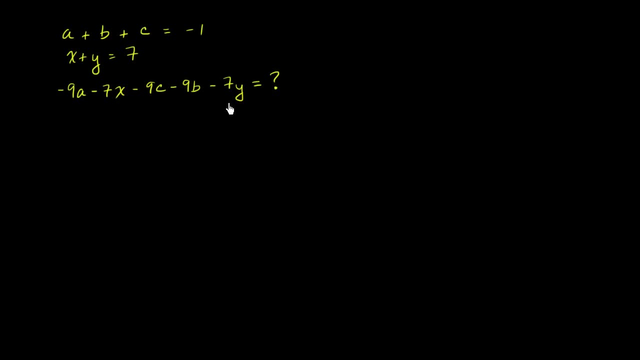 that x plus y is equal to 7, and then they ask us this big hairy thing: What is this equal to? And I'll give you a few seconds to give it a little bit of thought. Well, you could imagine they've given three variables, with one equation up here, another two variables. 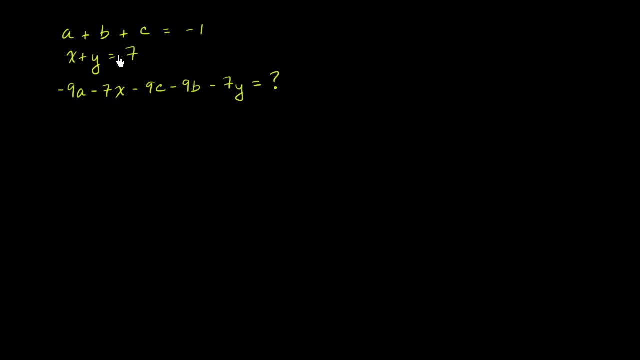 with another equation. We have five unknowns with two equations. There's no way we're going to be able to individually figure out what a or b or c or x or y is, but maybe we can use what we saw in the first equation. 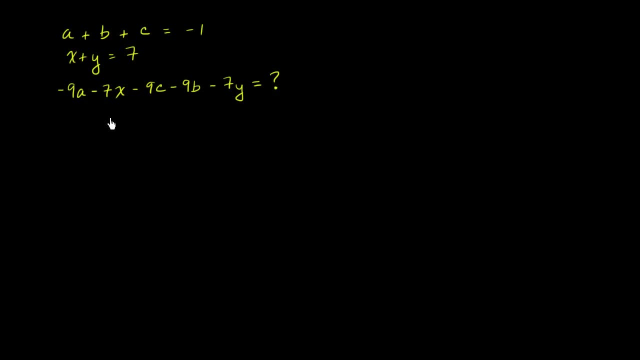 So what we saw in the last example to solve this, And so what we might want to do is rearrange it so that we have the x's and y's kind of grouped together and the a's, b's and c's kind of grouped together. So let's try that out. So let's focus first on the a's, b's. 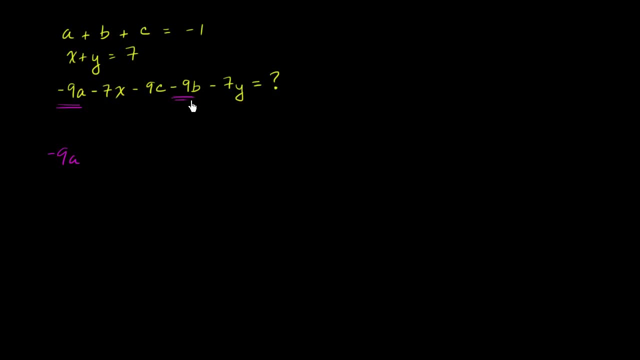 and c's So. we have negative 9a, negative 9b. I'll go in order, alphabetical order: Negative 9b and we have negative 9c And I think you see what's emerging. Negative 9c. And then let's work on the x's and the y's, And then we have negative 7x minus 7x. 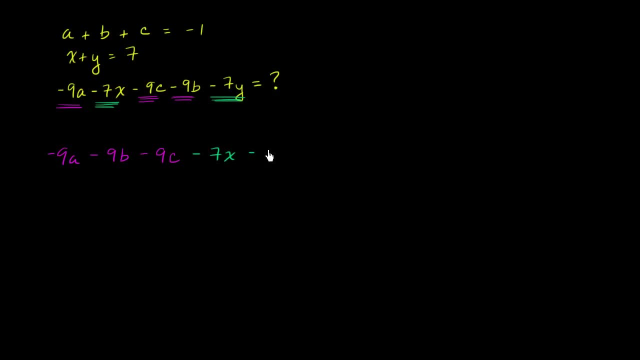 And then we have a minus 7y, So minus 7y. So all I have done is rearranged this expression here, But this makes it in a way, or it makes it a little bit clearer of what's going on here. These first three terms, I can factor out a negative 9. And I get negative 9 times. 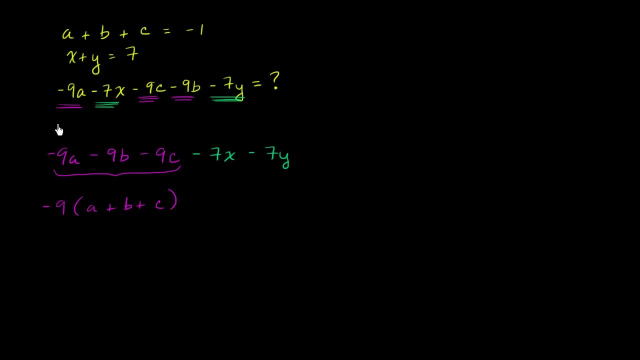 a plus b plus c And these second two terms, I can factor out a: 7. Minus, 7 times negative, 9 times x plus y. And just to verify, if you wanted to go the other way, multiply this negative 7 times x plus y. you'll get this: Multiply a negative 9 times a plus b plus.